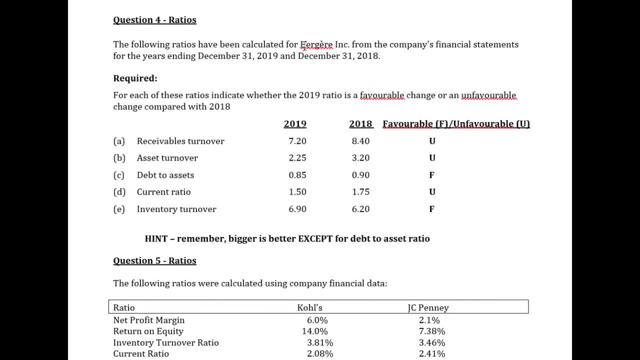 Here's a question on ratios, and this information has been taken from the statements of Berger for the years ending 2019 and 2018.. And we need you to tell us whether or not the change in the ratio is favorable or unfavorable to the company. So what you have to think about here is: if the ratio is increasing or decreasing, is that better or worse? If it's better, it's favorable. If it's worse, it's unfavorable. 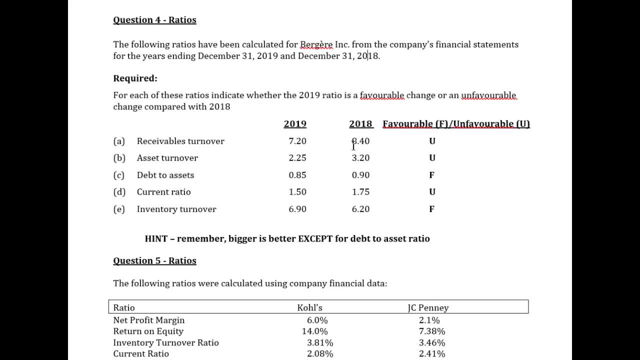 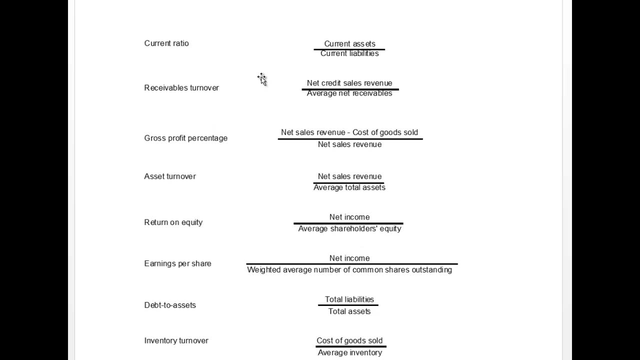 Then it's unfavorable, meaning that you have to know what the ratio means and how to calculate it in order to answer the question. So now what you will be given on the exam. these are the ratios you'll be given on the exam. Okay, so this is exactly how it will look. You'll get a current ratio and a formula, but you're not going to be told what it means. That's what you have to know. So you'll be given a whole series of ratios with a 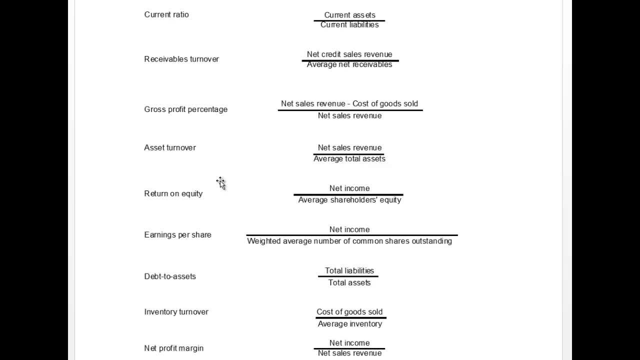 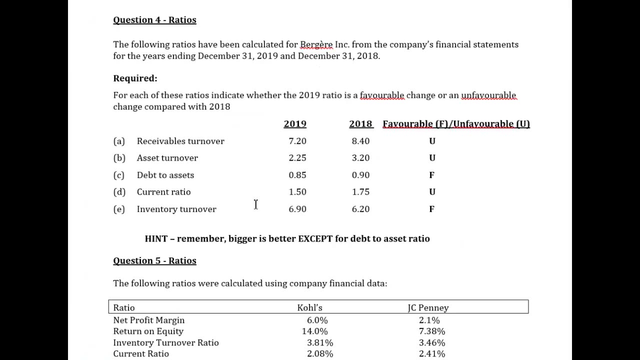 formula. So even in this question you don't have to calculate it. But what we find is that sometimes it helps students to see the formula because they can look at the formula and remember, through interpretation of the formula, what it means. So in our case, if we look at our question, the receivables turnover will tell us how much we're collecting in receivables in cash throughout the year. 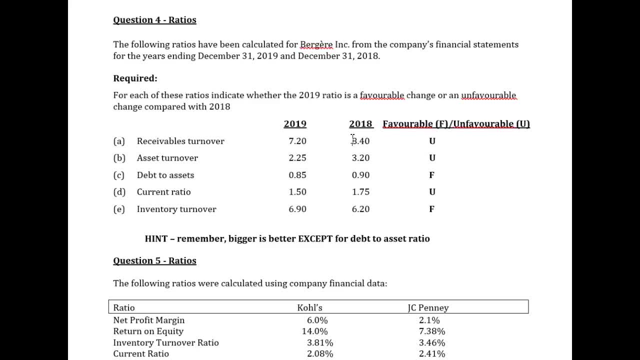 Right. How many times are we collecting? Well, we were collecting 8.4, or, say, on average, eight times a year. if we round it to the nearest whole time, Now we're only collecting approximately 7.2 times, or, say, to round it, seven times a year. Well, the more frequently we collect, it's better, right, But we're not collecting as much in 2019 as we did in 2018.. So that's unfavorable, Right. 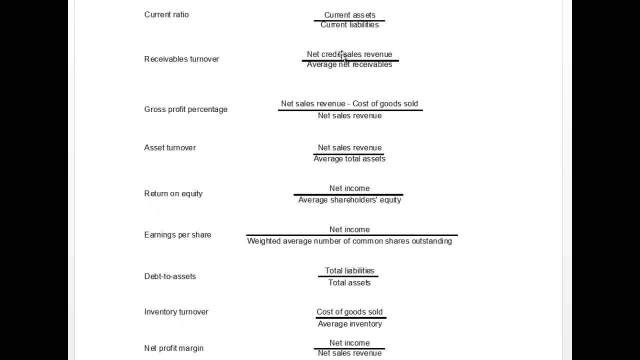 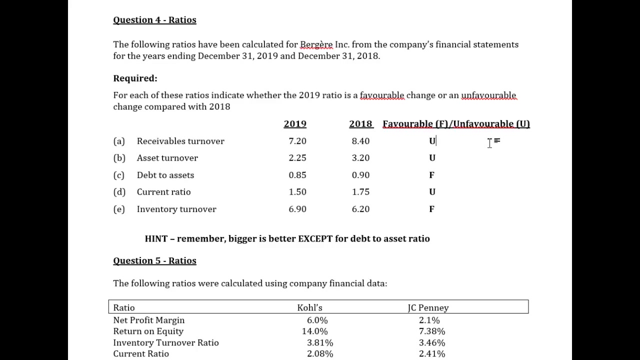 And you can see by the ratio right: Average net receivables based on credit sales revenue. So how often are you turning over those receivables that you recorded as sales revenue? Okay, So that means that in our case, because the number is getting smaller, you're not collecting as many times during the year, So that's unfavorable. Your asset turnover: That's a measure of efficiency of your asset turnover. 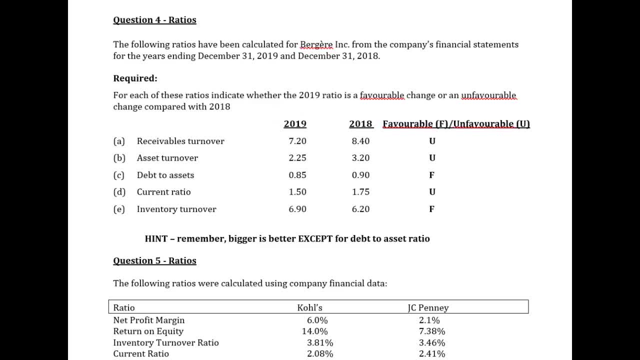 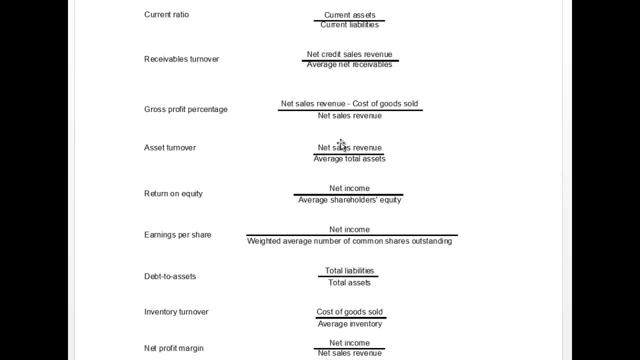 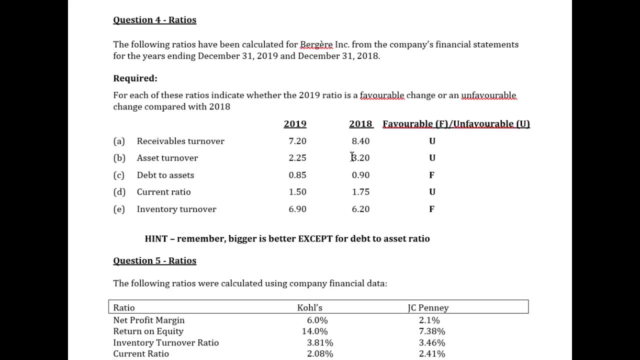 your assets to help you generate revenue. if you look at the formula, you can see that for all of our assets that we have, on average, how much sales revenue do they help us generate? so in our question, bigger is better. in 2018, we were generating 3.2 times in revenue the balance of our average total assets. now, 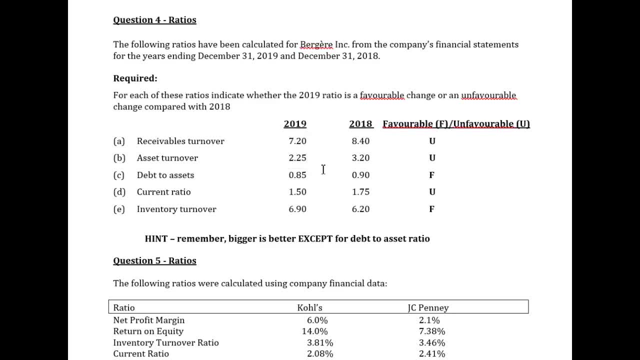 we're only generating 2.25 times the amount of revenue for the average assets we have, so that's lower. so we're not generating as much sales revenue as we were this year. we're not generating as much sales revenue this year as we were last year from our average total assets. so that's unfavorable, and don't forget. 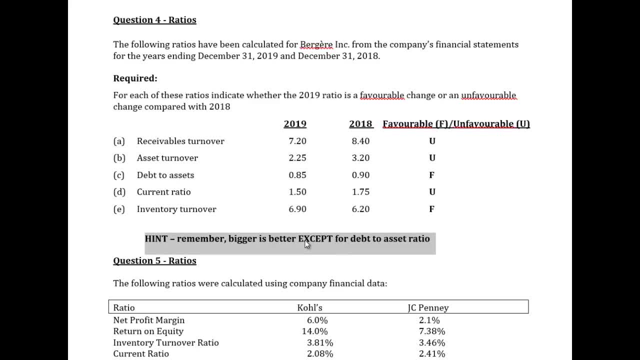 hint. bigger is better, except for that debt-to-asset ratio. all right now here. where is yule waiting? ok, let's try again. here, Yule waiting? this is when we come to the last time. all right now here. where is yule waiting? are at the debt-to-asset ratio. Debt-to-asset ratio is a measure of solvency. It measures 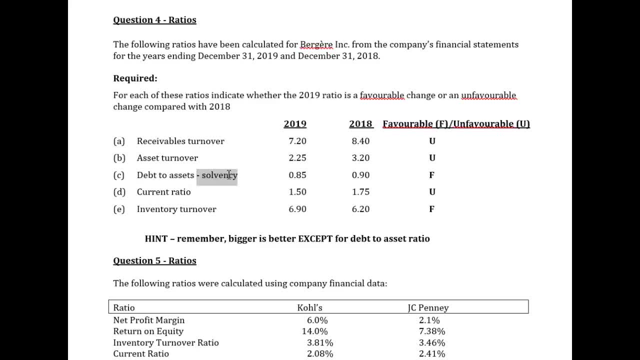 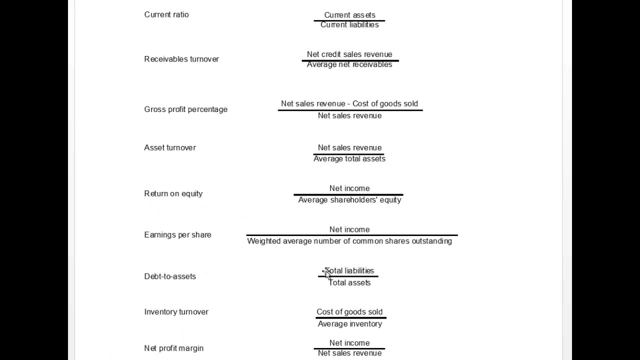 solvency. So in our case we want to know on a long-term basis how solvent is our company. All right, so we're going to look at total debt to total assets. So that formula here is total liabilities to total assets. So we want to make sure we're generating enough assets to clear off. 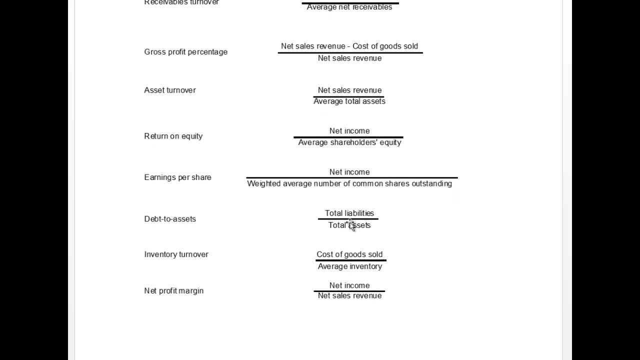 all of our liabilities, current and non-current. Well, you can see here that if we had more assets than we did, liabilities, that would be better. So the smaller the better here. So if we increase the denominator, that makes the whole fraction smaller, But if our liabilities are way bigger. 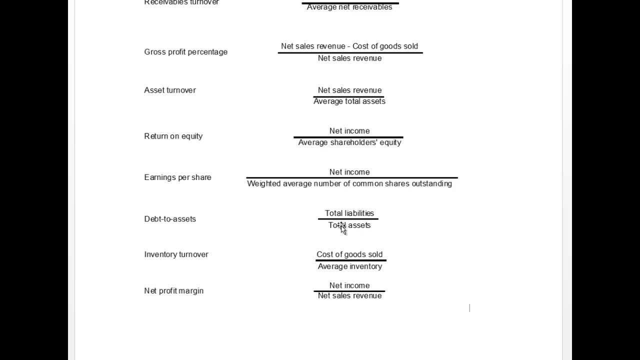 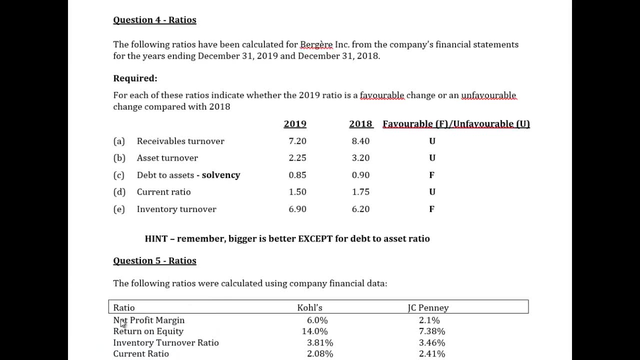 than our assets. that would be better. So if we increase the denominator, that makes the whole ratio bigger And that means we're not going to have enough assets to clear off all of our liabilities. So now we have to think. in this case, smaller is better. Remember: bigger is better. 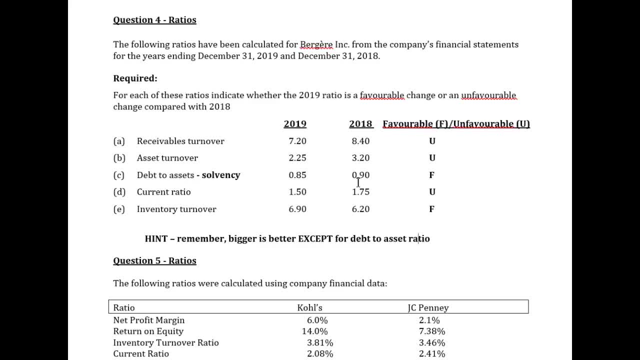 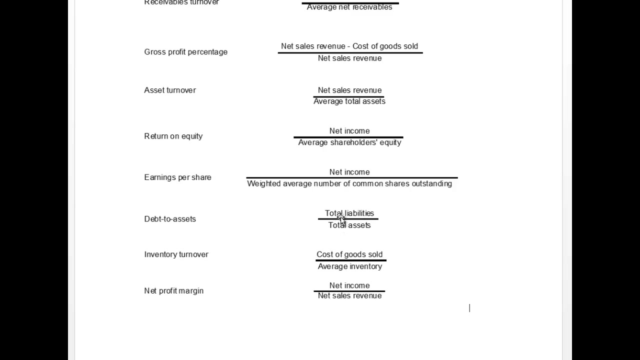 except for the debt-to-asset ratio. So what do we have? Well, it was 0.90.. So that means we had 0.90. So we had total assets. if you look at your formula right, We must have had total liabilities which were less than total. 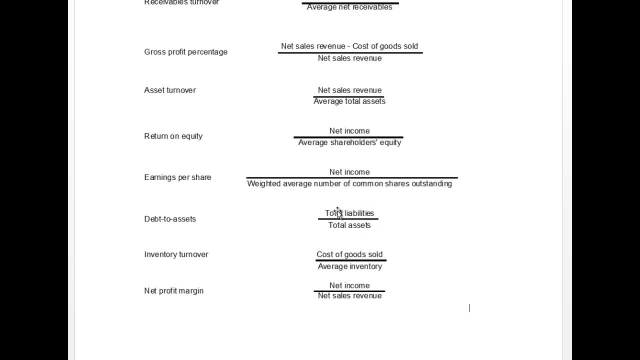 assets. So this ratio was 90%. So it means if it's greater than 1, it's not so good, right, But the smaller it is the better And it's less than 1.. So for every $10 in total assets, we had $9. 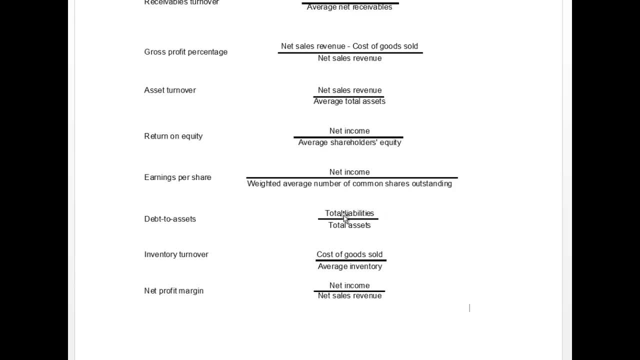 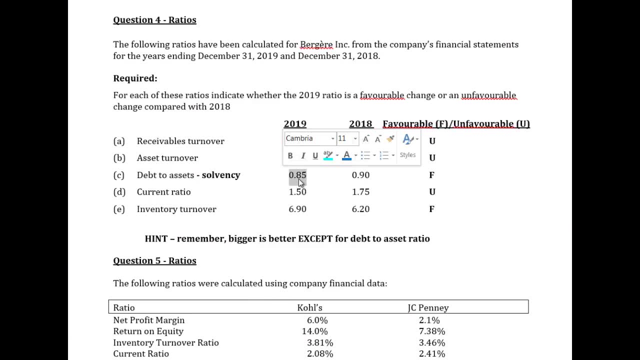 in liabilities. So if it's below 1,, the smaller the better. That's okay, That's not bad, But is it an improvement? okay, this year? Well, it's 0.85.. So that means that our liabilities are less than our assets. 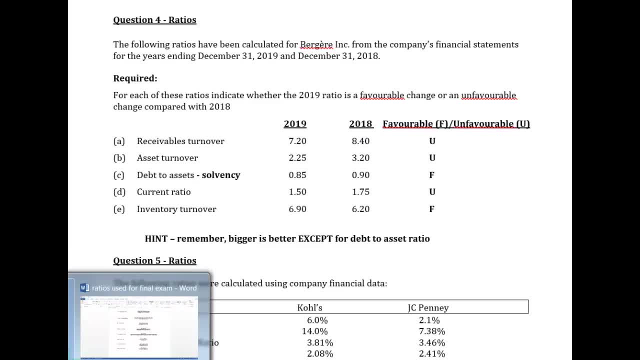 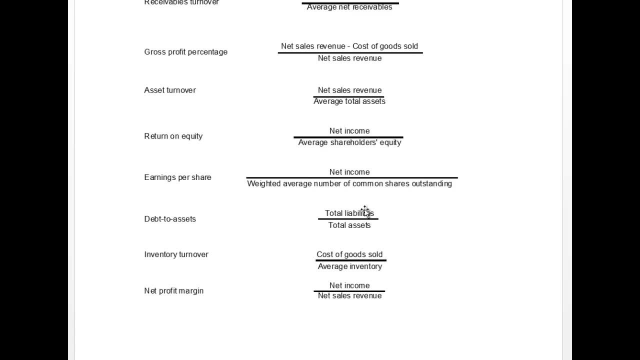 in an even better position. So if you look at your formula, that means for every, say, $10 in assets, you only have $8.50 in liabilities, right? You have less liabilities for the same number, right? So that means that we have a lot of assets. So in our case we would say that's favorable. 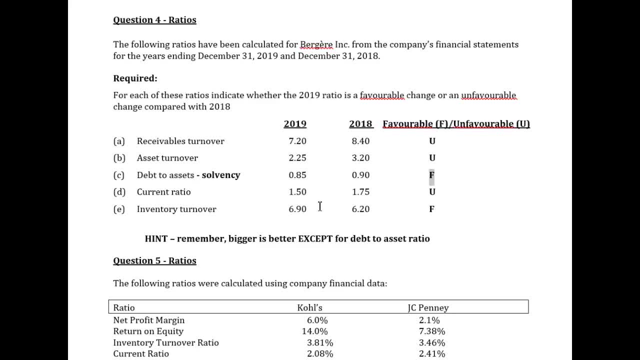 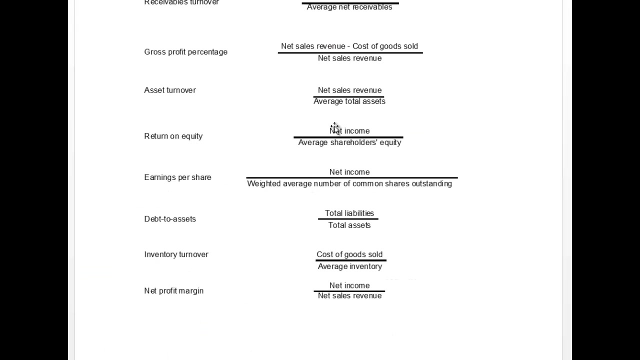 because as it gets smaller, it's better. Now, if you look at the current ratio, that tells us on a short-term basis how solvent we are on a short-term basis. So do we have enough current assets to cover our current liabilities? So if we have a look at our formula, you can see our current liabilities. 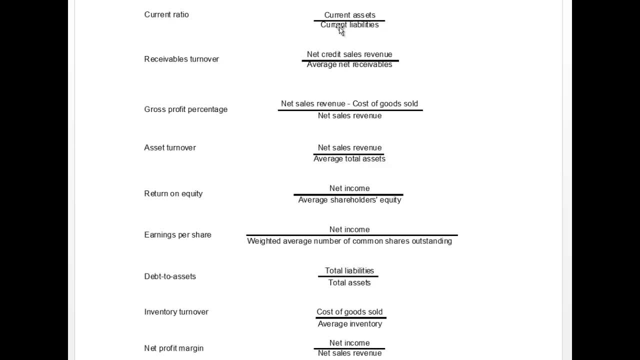 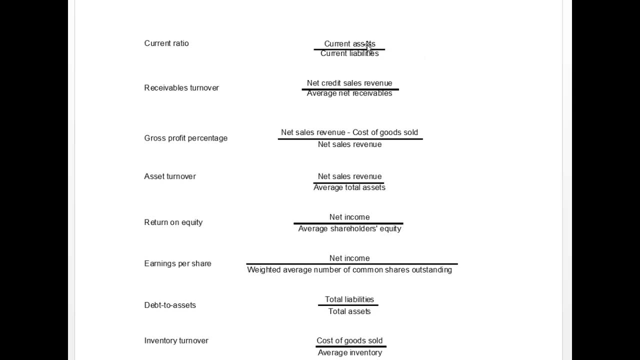 Our current ratio looks at current assets to current liabilities, So the bigger this ratio is the better. Why? Because that means our assets get bigger than our liabilities, which is what we want. But we're talking about a current ratio, so we're looking at current assets divided by current.